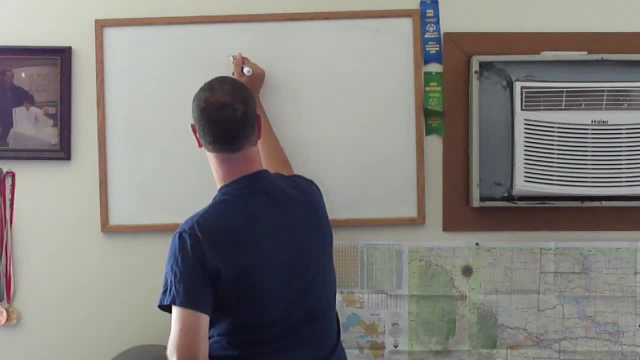 Let's go, 758. And we'll take away 416. What's all of that? 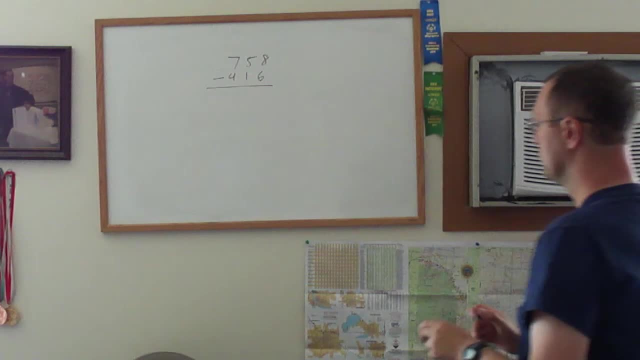 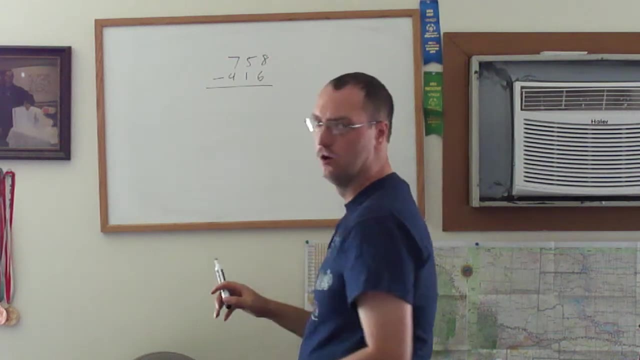 No. All the numbers on the top are bigger than the numbers below, so we're not supposed to do borrowing or anything right at this moment. 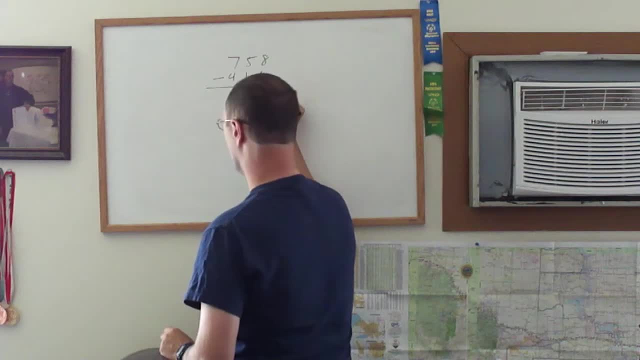 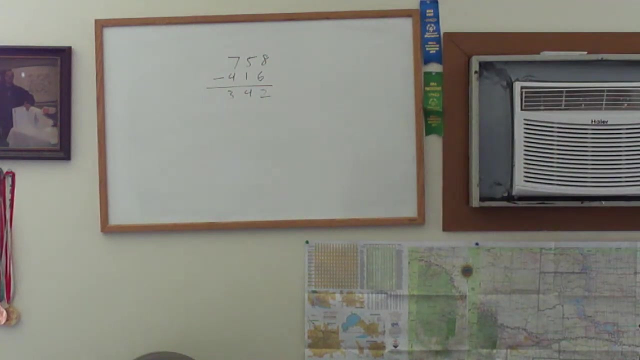 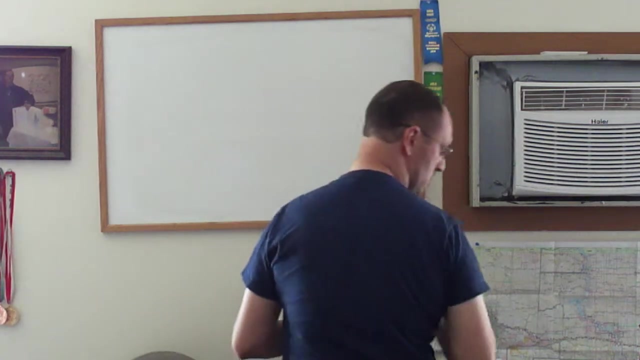 So 8 minus 2 is 8, no, 8 minus 6 is 2, 5 minus 1 is 4, and 7 minus 4 is 3. 342. But let's try, let's do one more, let's do one more of that before we get to the borrowing, before we get to the borrowing. 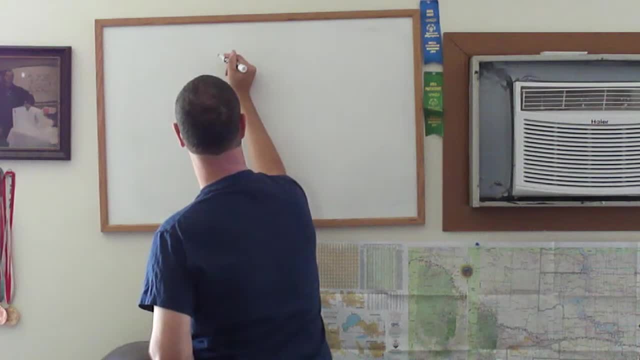 Let's go with 48,783. 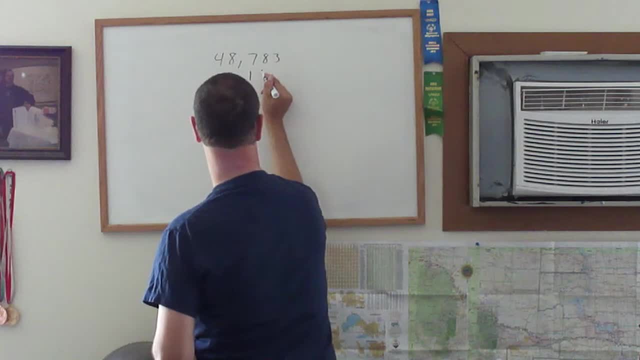 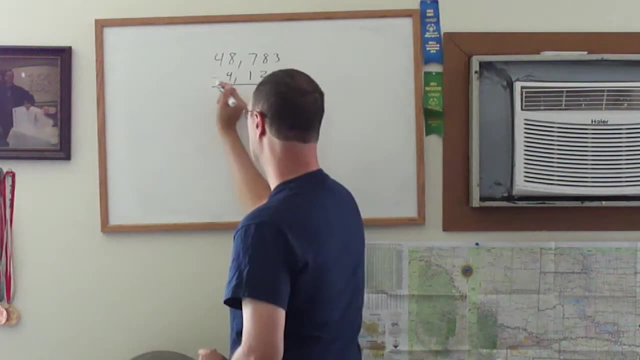 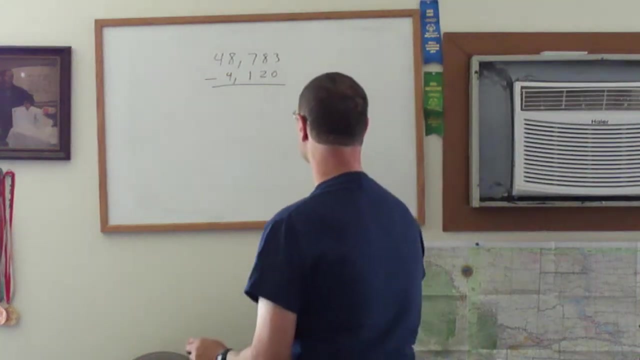 4,183. 4,183. 4,183. 4,183. 4,183. Well, I'll take away. Now here, no borrowing this time. 4,183. 4,183. 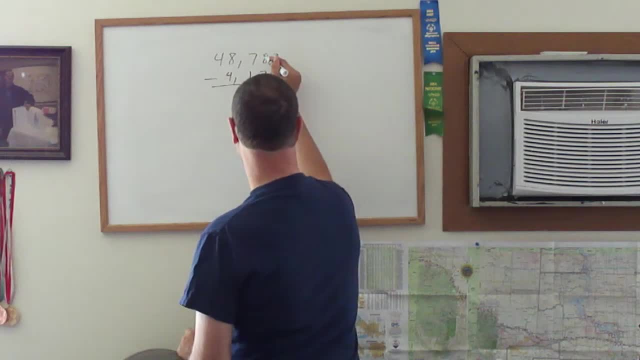 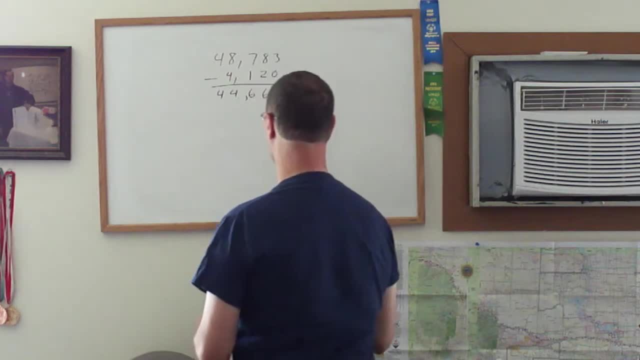 If 4 and 0 is just 4, it's 44,663. 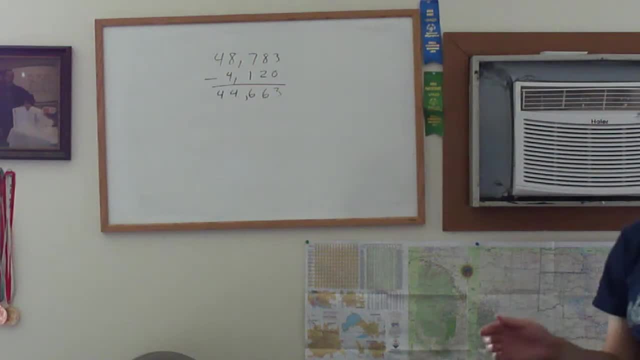 Can you get the idea of how to subtract whole numbers now? Alright. That's how you subtract whole numbers. 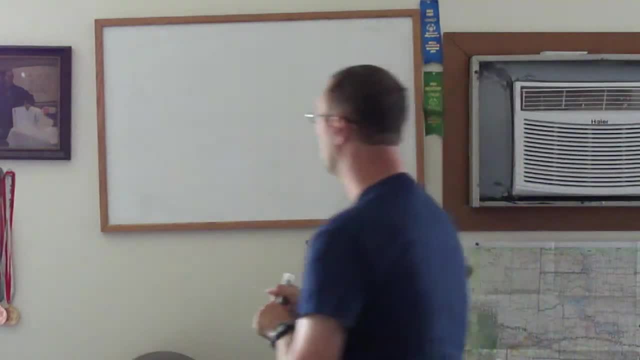 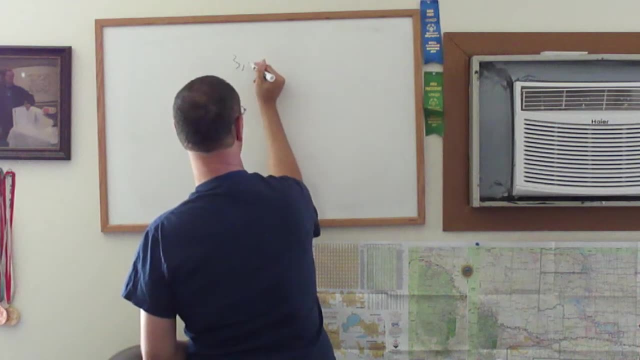 Now, let's get a little tougher. Let's go with 3,715 minus 1,290. Alright, a little tougher there. 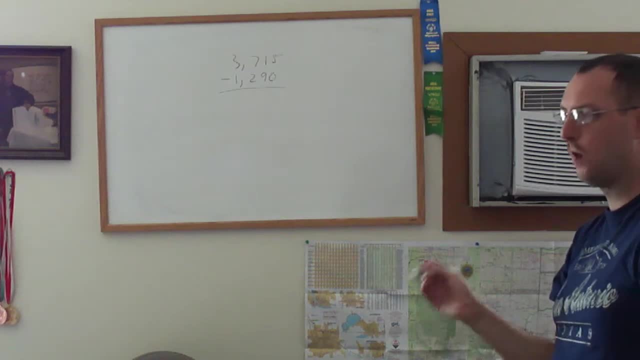 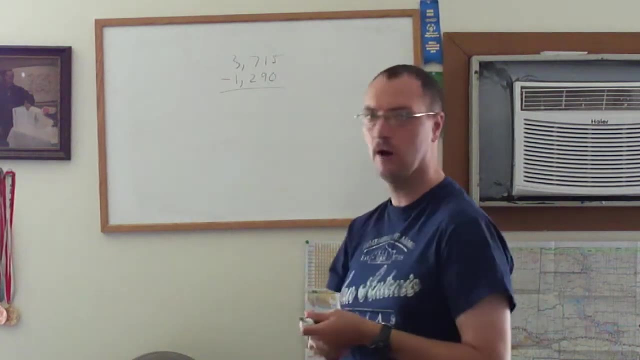 What is borrowing? Let's find out. What is borrowing? Now we're going to talk about borrowing or regrouping. 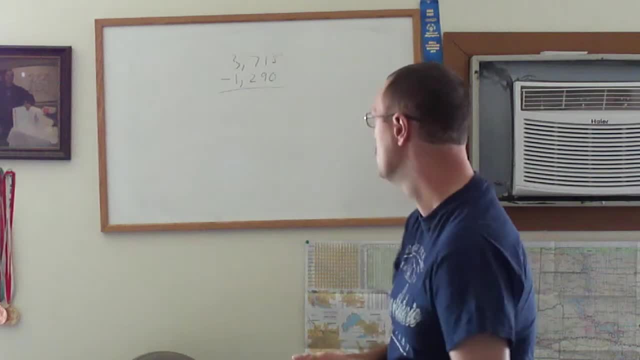 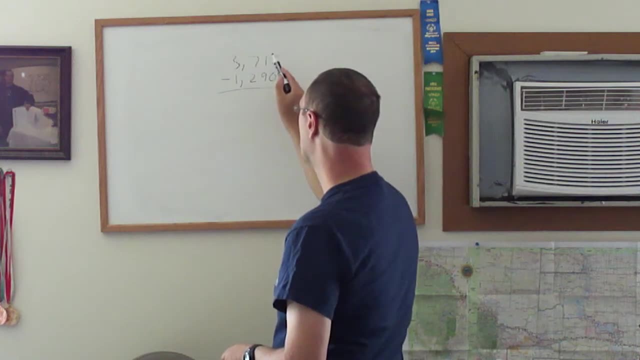 Borrowing is the terminology to take one number, take the number on top and borrow the one, on the other side. 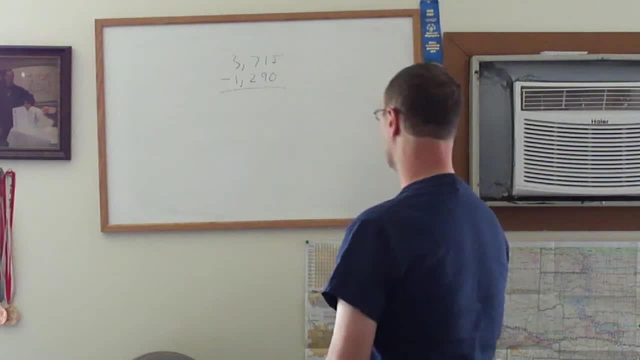 Let's put that in action. 5 minus 0, well it's just 5. 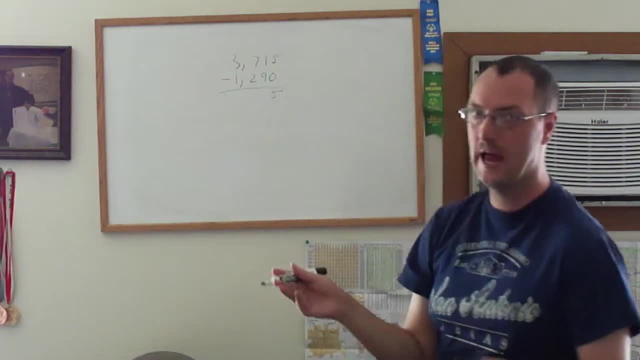 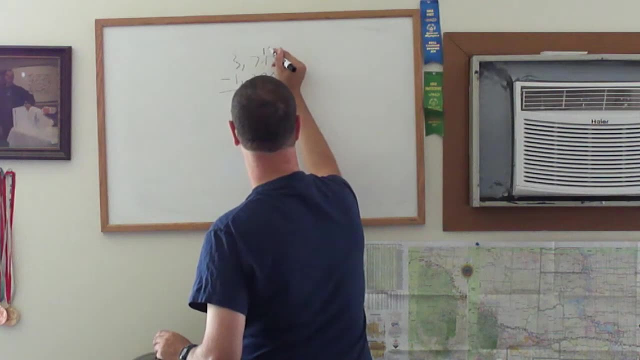 Now, 1 minus 9, we can't do that. So now, we're going to borrow. Make that an 11. And we're going to borrow the 7 to a 6. 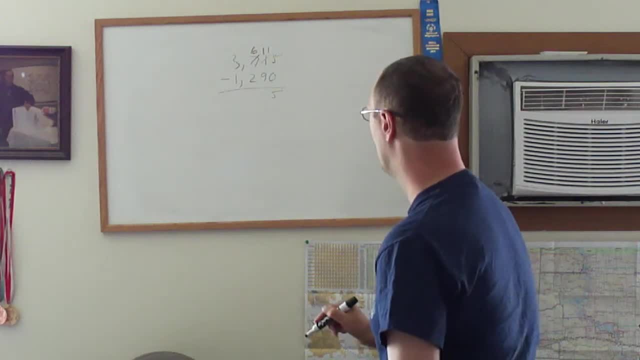 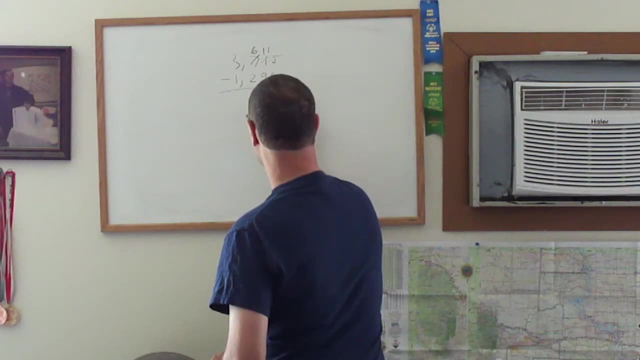 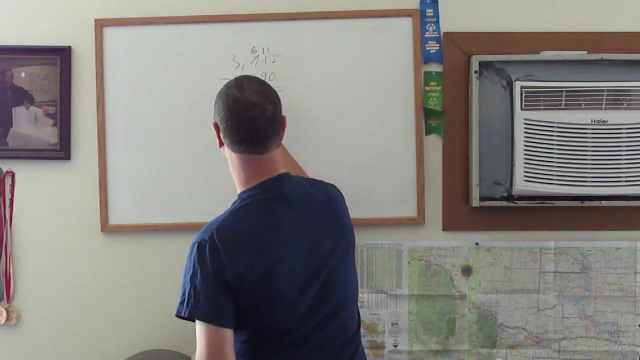 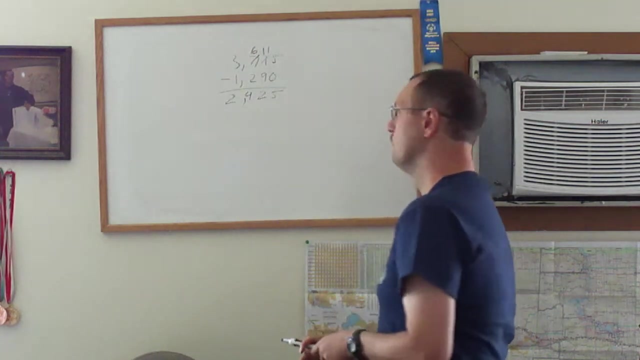 Alright, 11 minus 9 is 2. 6 minus 2 is 4. And nothing right there. 3 minus 1 is 2. That's how borrowing works. 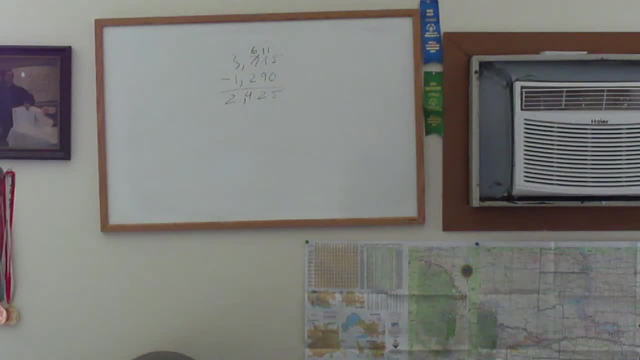 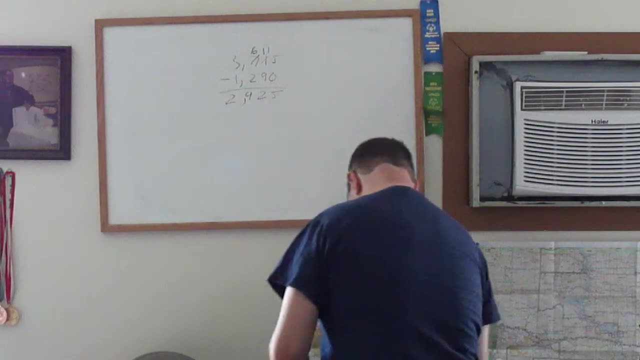 I'm going to use different hands this time. I'm going to use purple this time. That's how borrowing is. So let me put that in the definition. 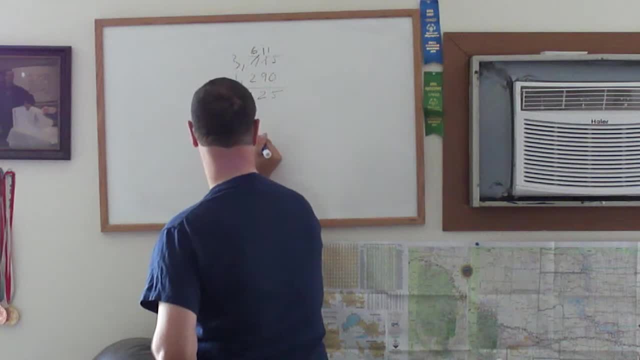 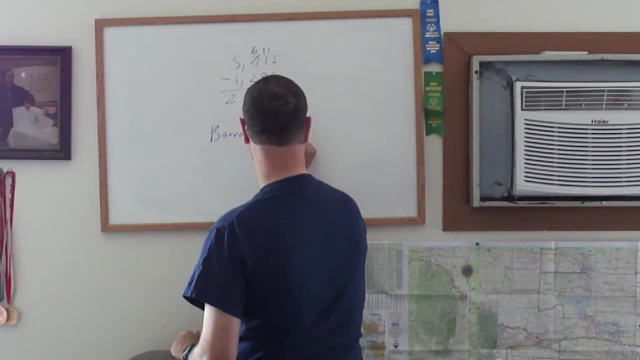 Borrowing is to find a, taking a 1, taking a 1, on one side, on one side. 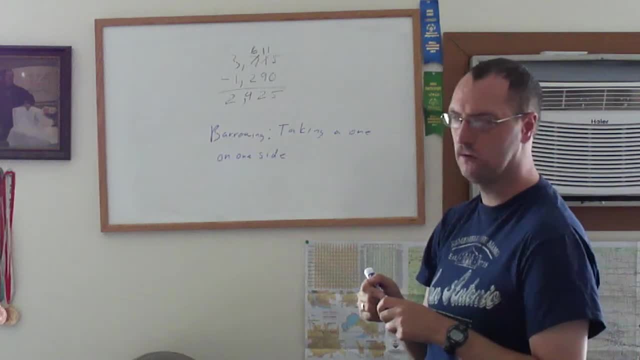 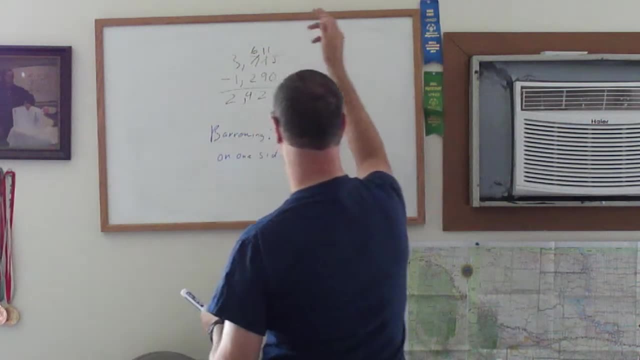 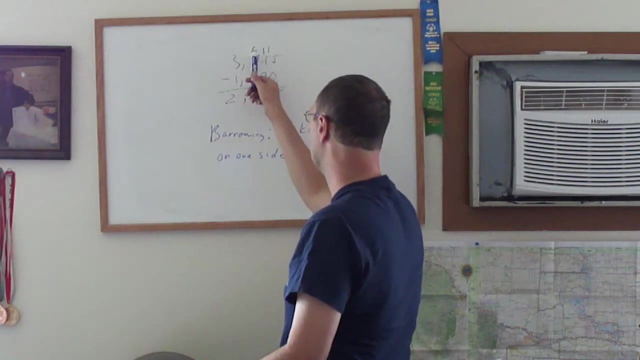 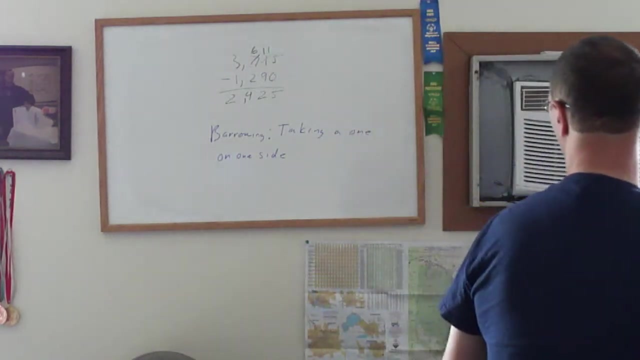 And that's how, that's what borrowing basically is. It's taking a 1 of a number, taking a 1 of a number on one side. So we're taking a 1, taking a 7, taking a 1 on the left side, making it 11 on that right side. 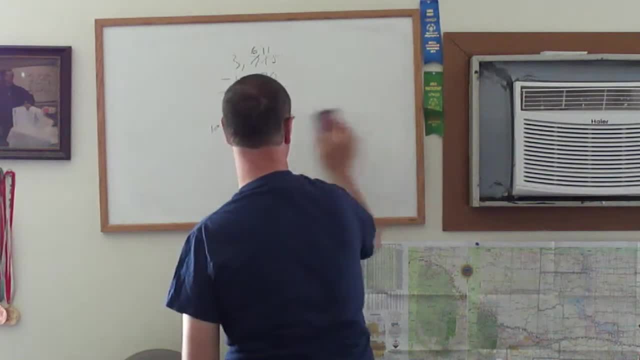 Now let's try, now let's try something a little tougher this time. 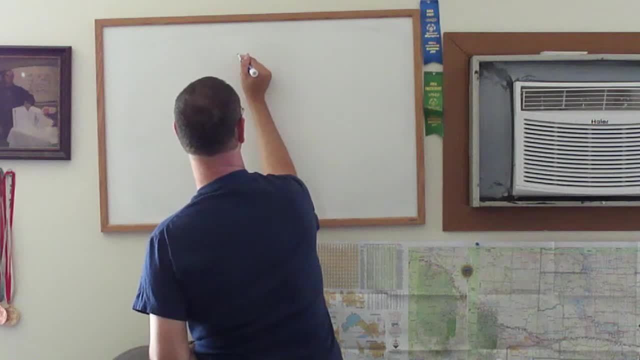 Let's go with, 53,920 minus 18,474. Alright. 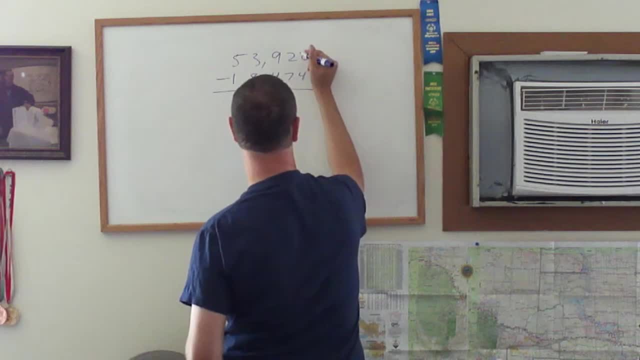 Again, borrowing will it take, it can. Alright. 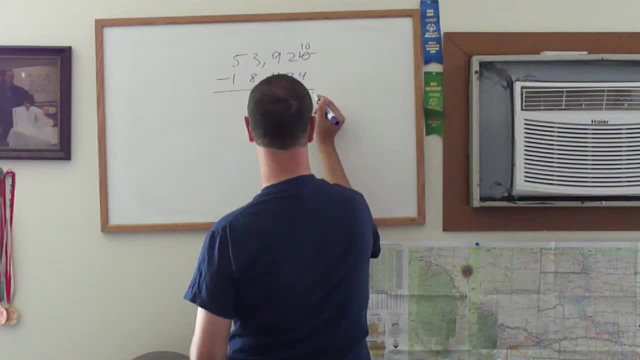 And we're going to subtract it from 4, making it a 6. Well, well we can't, well we're going to take that number, 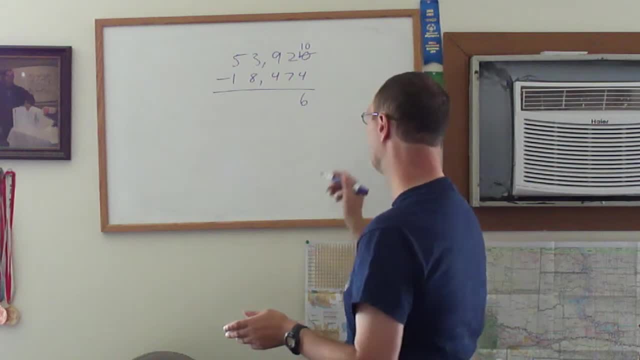 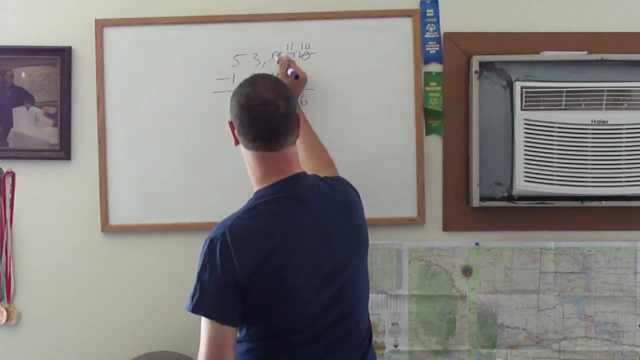 but we can also subtract 2 from 7. So we're going to borrow one more time, but we're going to make this a 11. And subtract it from there, 11 minus 7 is 4. And we're going to subtract mid, making it an 8. 8 minus 4 is 4, comma. 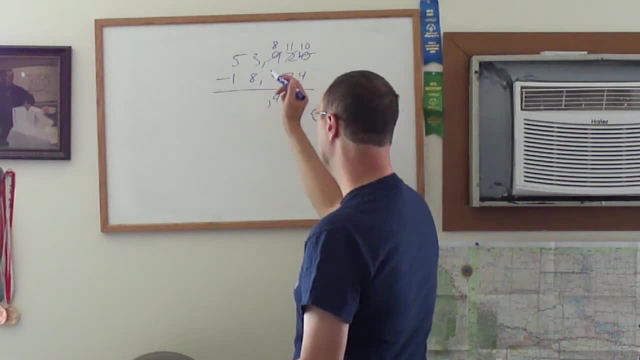 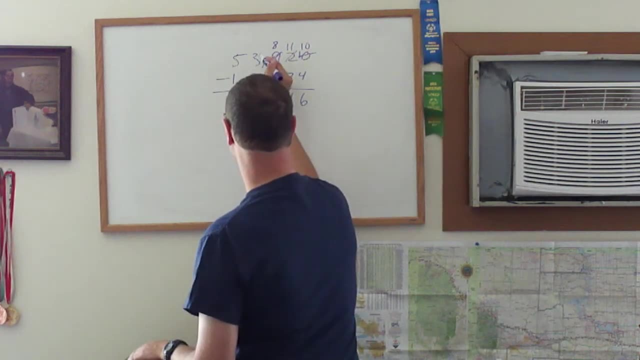 And we can't subtract 13, 13, not 3 from 8, no, yeah, we want to make it a 13. So subtract it from there, we get 5. 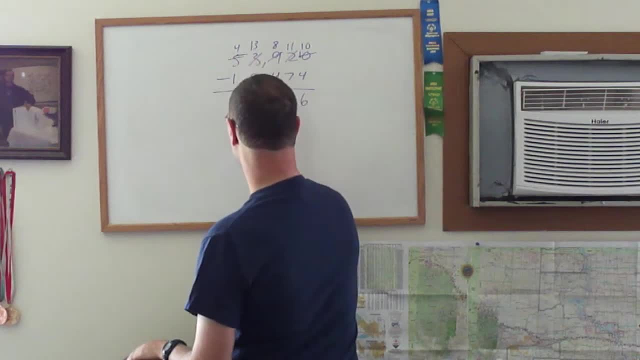 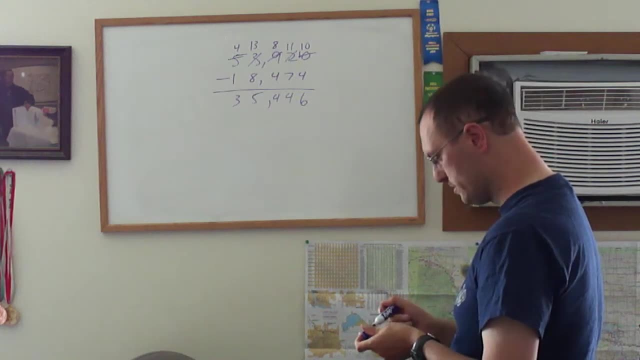 Make it a 4. 4 minus 1 is 3. So we got the answer, 35,446. 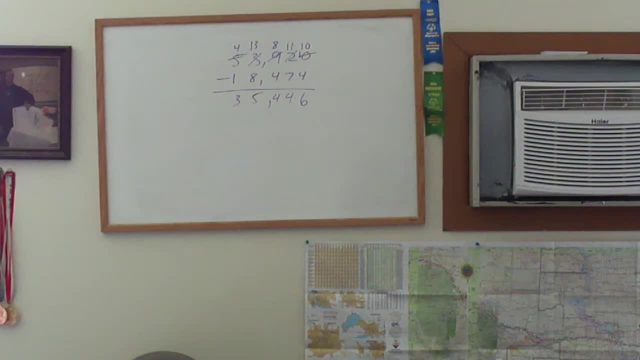 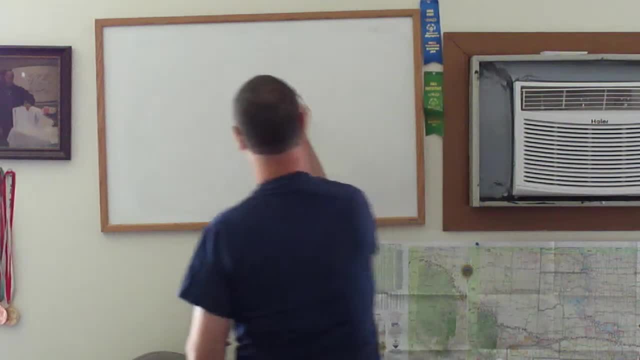 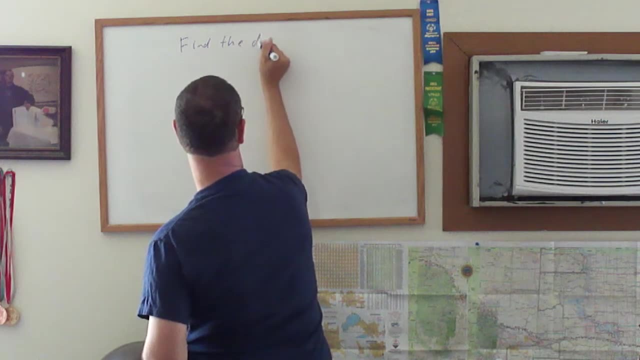 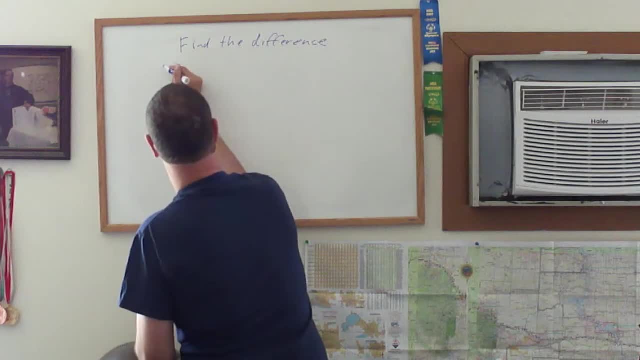 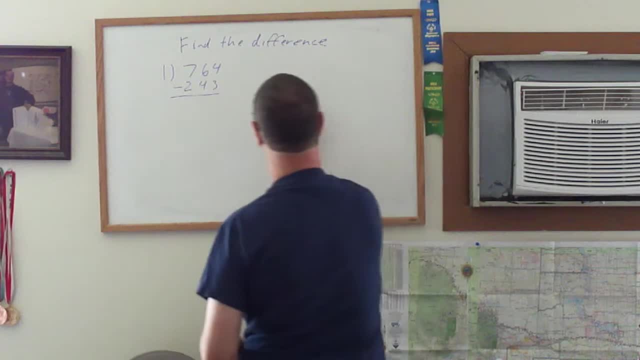 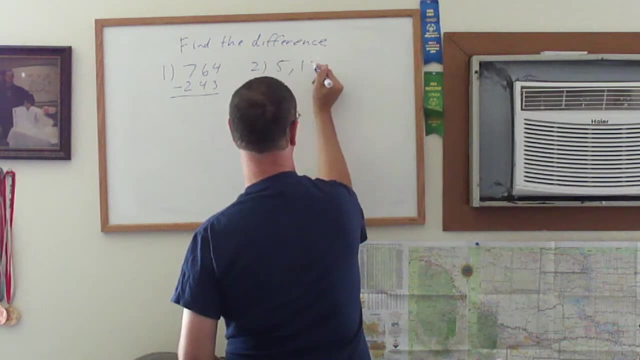 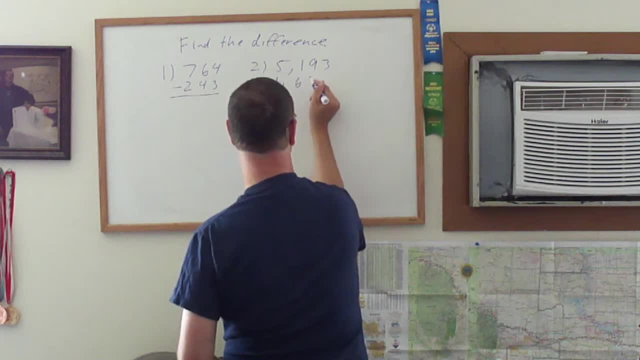 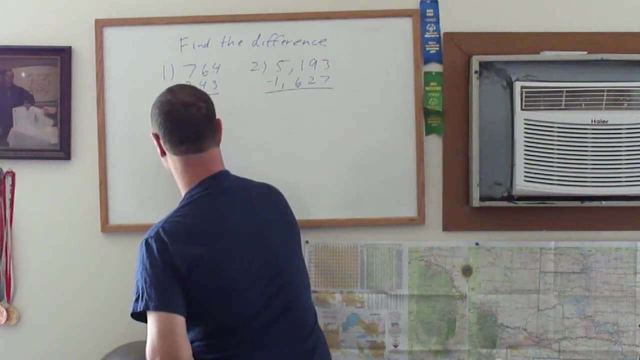 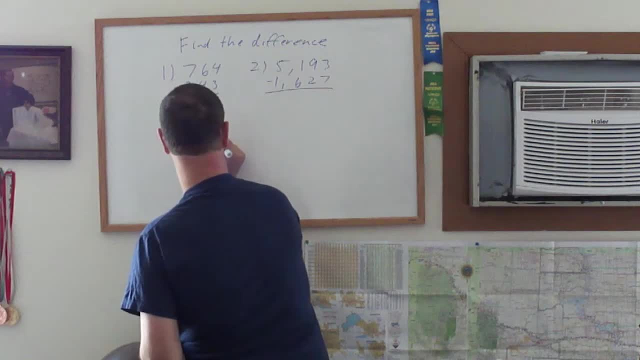 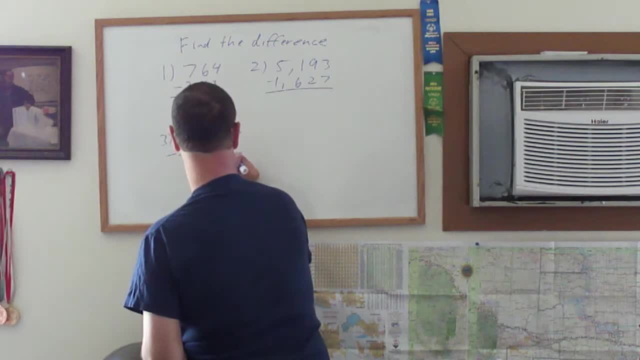 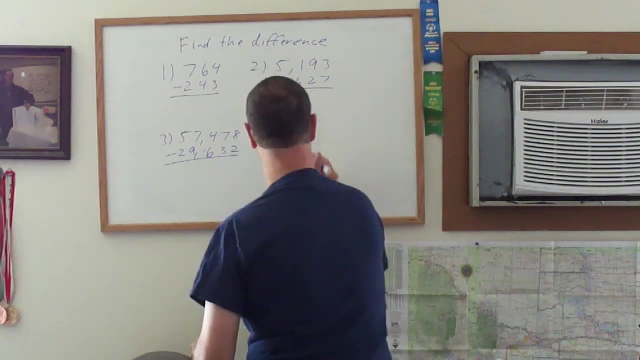 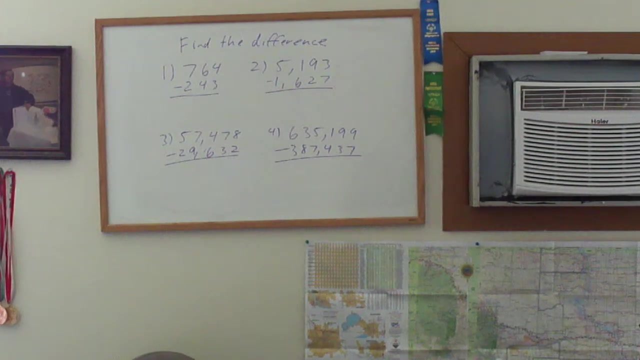 1, 1, six hundred thirty-five thousand one hundred and ninety-nine minus thirty-eight thousand three hundred eighty-seven thousand four hundred and thirty-seven that is included for today 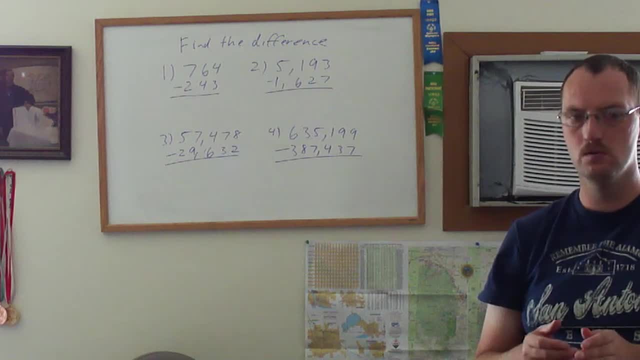 and tomorrow's lesson we're going to introduce what multiplication is and how to multiply. Thank you. Thank you.